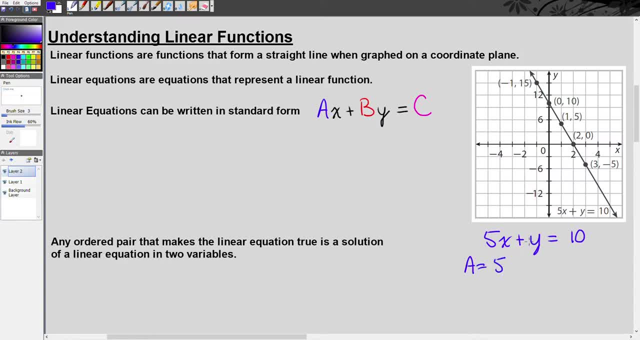 value is 5.. Our b value is the invisible number 1 here in front of y. It's a coefficient of 1. And our c value is 10.. Now you need to be able to identify from an equation whether or not it represents a linear. 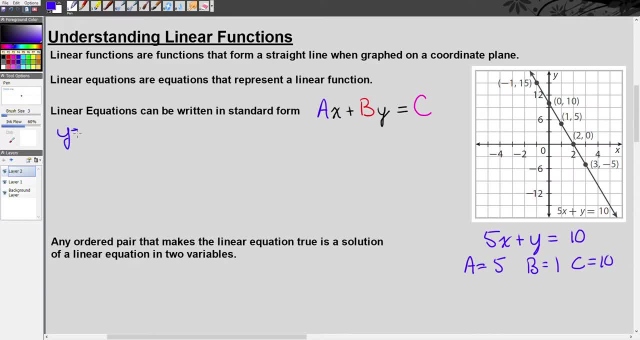 function, And that's actually quite easy to do. Any linear, any equation that can be written in standard form- ax plus by equals c- is a linear function. So, for example, if I have the equation 7x minus 2y equals 5.. 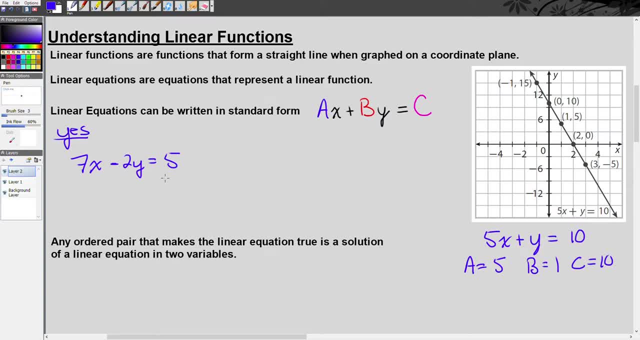 This is a linear equation. This is a linear function because it is written in standard form. Okay, I could even have standard form if I have fractions, your favorite thing, Correct? So if I have here, for example, half x plus two-thirds y equals negative 4.. 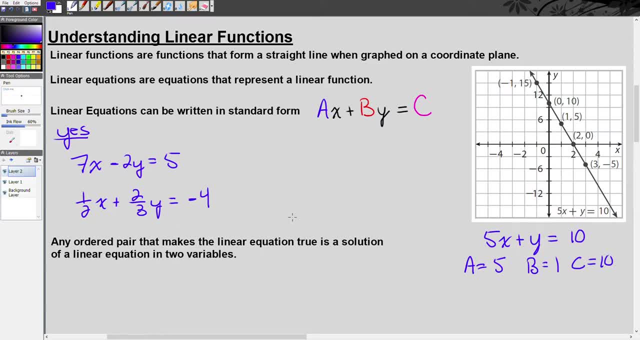 This is also a linear equation. It represents a linear function. So what are the no's? Okay, What are the? what does a no look like? An equation that is not a linear function? Well, if your equation has an exponent other than 1 on any of your variables, 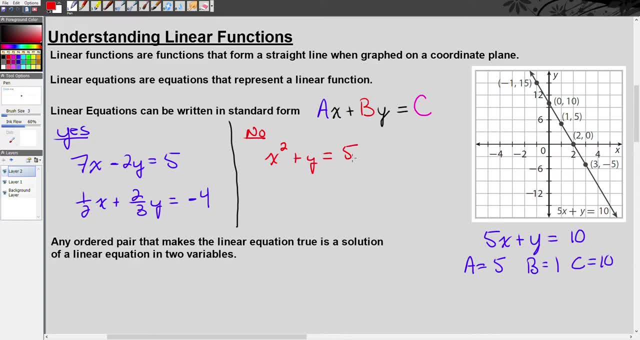 then it is not linear. So, if I have your x squared plus y equals 5.. Okay, This is not a linear function. It may still be a function, but it's not linear. And what makes it not linear is this exponent of 2 here. So remember the rule is: 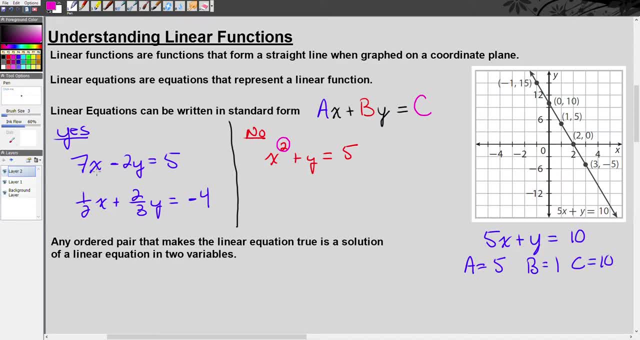 if any of the variables have an exponent other than 1.. Because if you look back over here on the yes side, these x's and these y's, they do have an exponent. It's the invisible 1.. Okay, So these are okay. 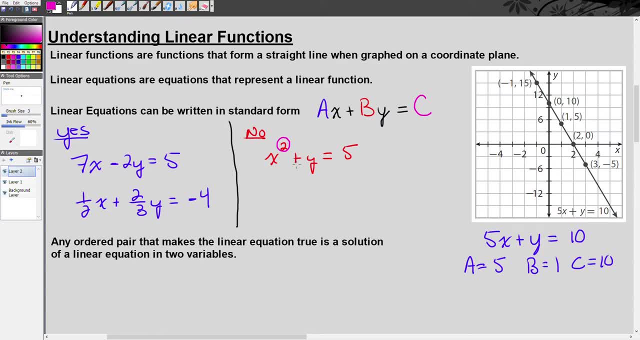 It's when the exponent is other than 1. Then it is not a linear function. What else would not be a linear function? It would be if your either one of your variables, x or y, is the denominator of a fraction. So I might have here: 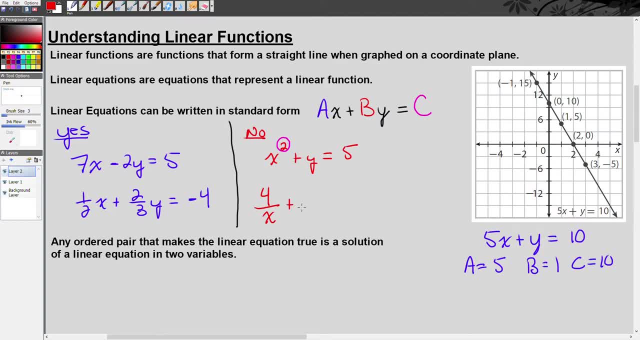 4 over 1.. x plus 3y equals 10.. This is not a linear function because x is a denominator for that fraction, So this would not be linear. okay, So that's how you can identify a linear equation from a non-linear equation. okay, So next part here. any ordered pair that 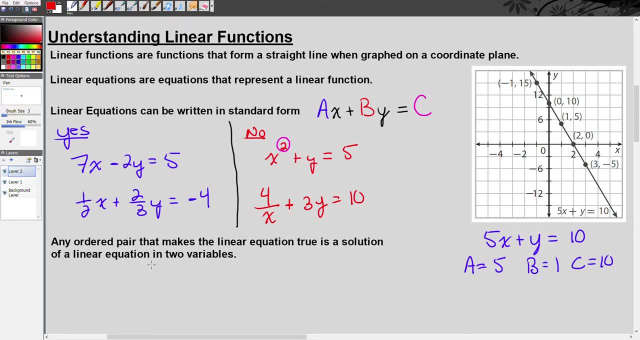 makes the linear equation true is a solution of a linear equation in two variables. This in two variables is because, remember, we do have two variables here. We have x and we have y. So what does that mean? Well, if we take a look here at this graph, you see it lists some points here. for 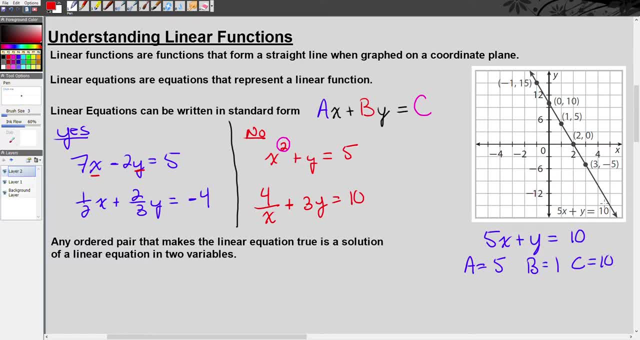 us. All of these points are on this line because they are solutions to the equation: 5x plus y equals 10.. That means when you plug in the x and the y value into this equation, okay, for any one of these points you're going to get a solution. So if you plug in the x and the y value into this, 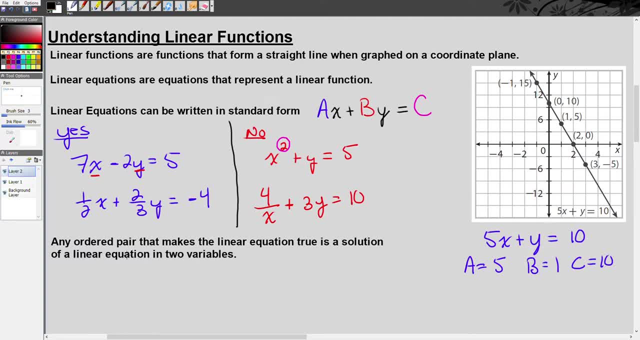 statement, you're going to get a true statement. So, for example, if I do one here, so I have here 5x plus y equals 10.. Let me scroll down a little bit, okay, Then I'm going to pick this point here. 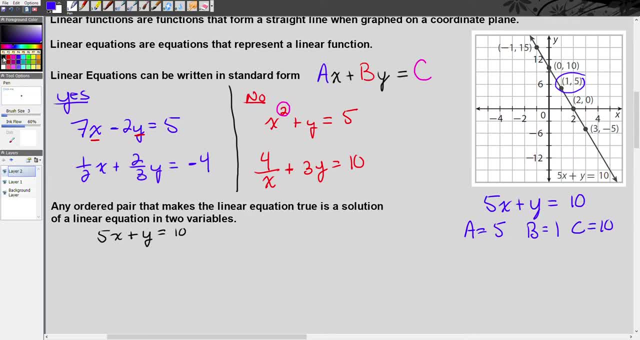 1 comma 5.. And I strongly recommend, whenever you're substituting for variables in an equation, to use parentheses. So I'm going to say: 5 times whatever x is plus whatever y is equals 10.. And I'm going to substitute in here a 1 for x and a 5 for y. So now, what is 5 times 1? 5? 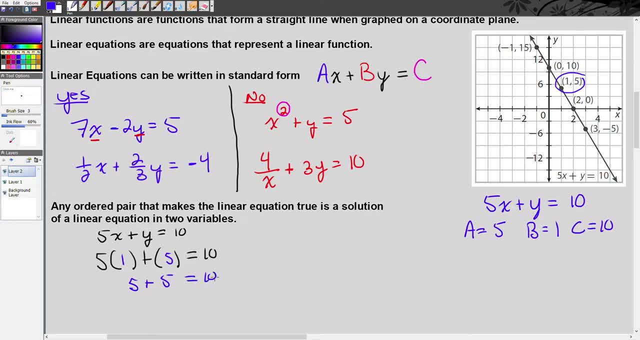 plus 5 equals 10.. Is that true? Yes, Let's try another one. So again, 5 times: whatever x is plus whatever y is equals 10.. And let's go ahead and see. Let's pick here this point. 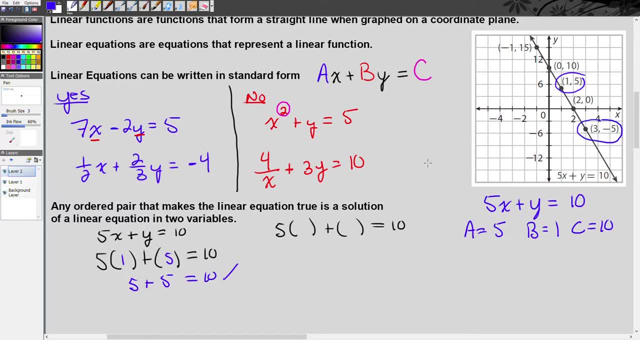 3 comma, negative 5.. Okay, so I'm going to substitute 3 for x and negative 5 for y. And let's work it out: 5 times 3 is 15 plus negative 5 is the same thing as just saying minus 5.. And is 15 minus 5 equal to 10? Yes, it is, That is true. 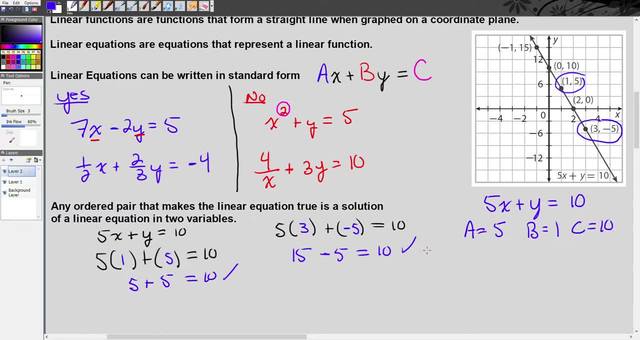 So you can see how those are solutions for the equation And any point that I were to choose on this line and substitute the x and y values, I would get a true statement. Even if I were to pick one of these in-between points Now it would be difficult to do because I would have to know. 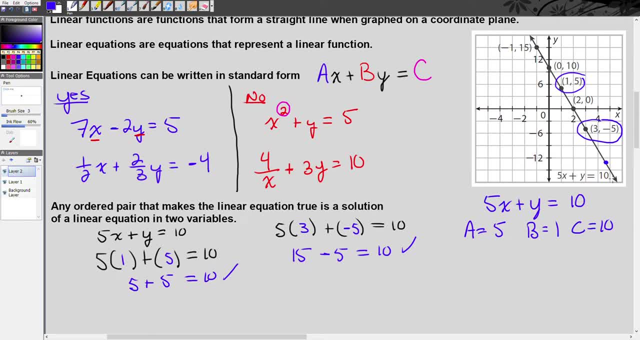 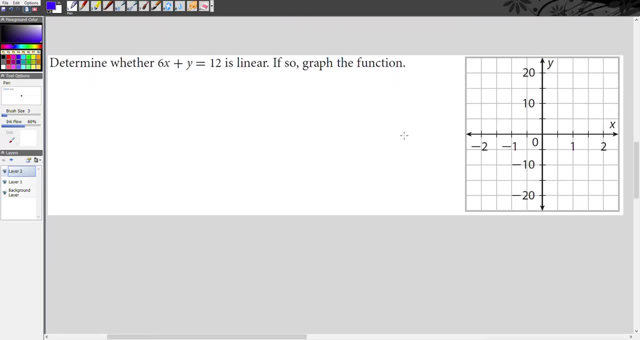 exactly what the x and y values are for that, but it would work. Okay, All right. Next part of this: Take a look at this question here. Determine whether 6x plus y equals 12 is linear. If so, graph the function. Well, is it linear? Let's take a look. Do either of my variables have an? 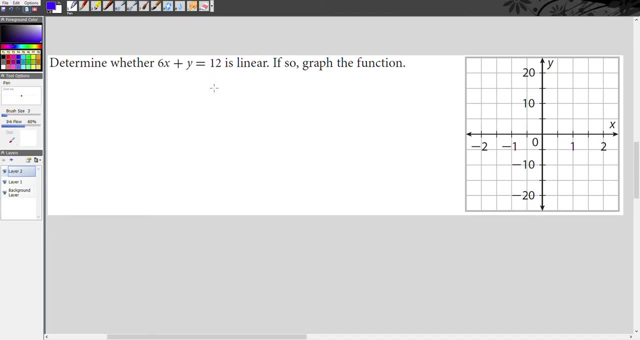 exponent other than 1?? No, Are either of my variables the denominator of a fraction? No, So is this a linear function? Yes, it's a linear function. Okay, So now let's graph it. What are we going to do? Well, we're going to make a table, Very simple table here x. 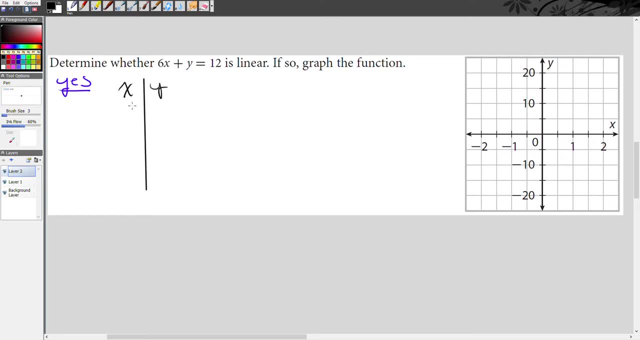 and y. Okay, Now I'm going to. first I need to take this equation here: 6x plus y equals 12, and I need to solve it for y. Remember that means that I need to get y. 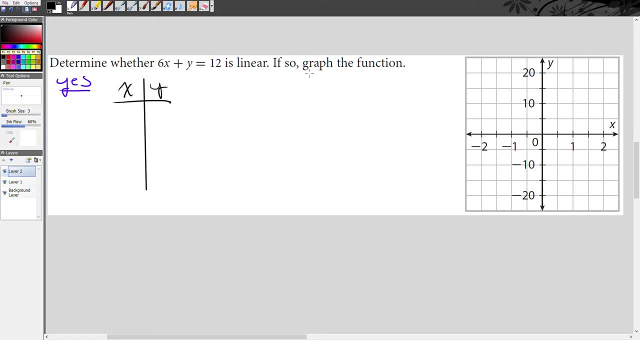 and I need to get rid of 6x from this left side here. So if we do that over here, real quick: 6x plus y equals 12.. How would I get rid of that 6x? Well, I have to subtract 6x from both sides. 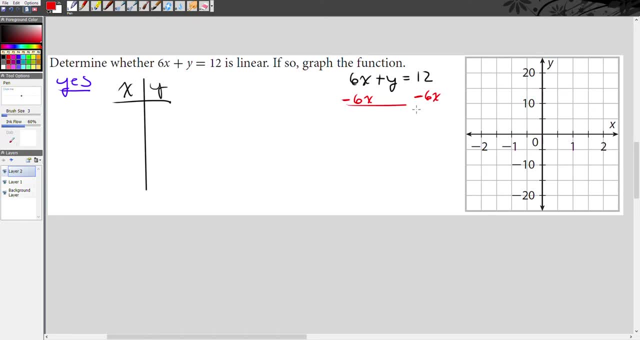 right, And I end up with the equation: y equals 12 minus 6x. So now this is going to be easier to do. So what I'm going to do is I'm going to choose a value for x. 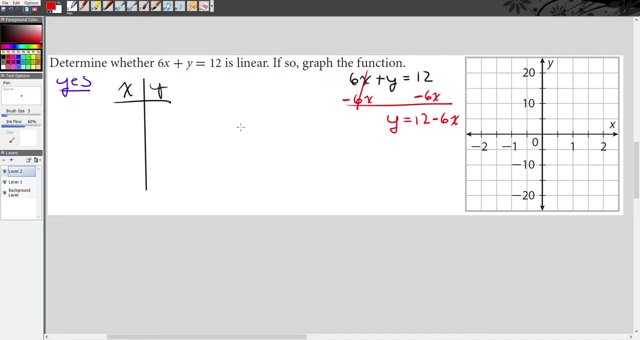 substitute it and see what the y value comes out to do. And where can I get my x values? Well, look at the graph. here. I have a negative 2, a negative 1, a 0, a 1, and a 2.. So let's use those. 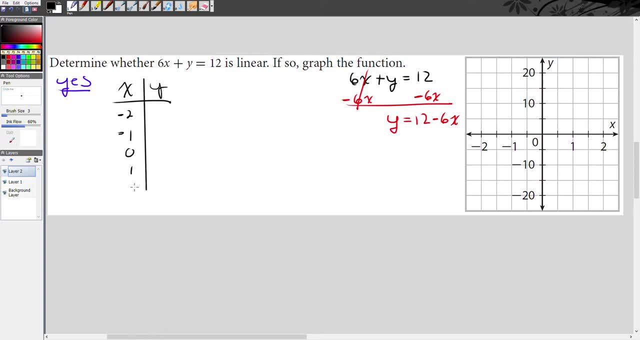 Negative 2, negative 1, 0, 1, 2.. Okay, And so let's go ahead and substitute. So, starting with negative 2, I'm going to say here, let me start up here: y equals 12 minus 6 times x. 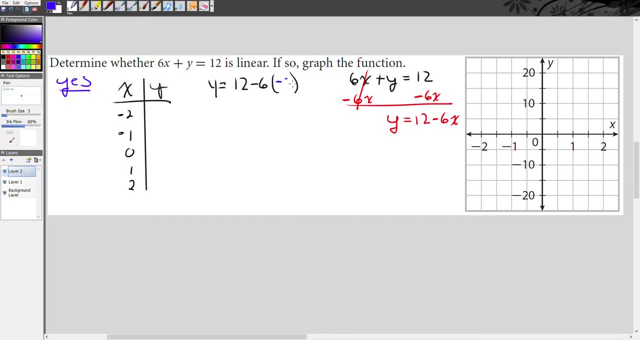 So this time x is negative, 2. And now negative 6 times negative. 2 is positive, 12. And 12 plus 12 is 24.. So y equals 24 when x is negative 2.. Now we do the same for 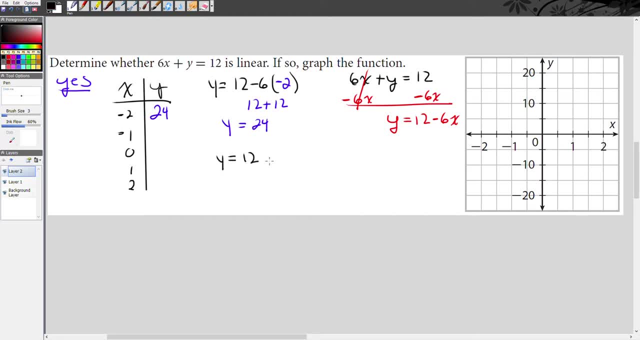 negative 1.. So again, y equals 12 minus 6 times 1.. Negative 6 times 1 is negative 6.. And 12,? well, sorry, it's negative 1, right? So this is going to be positive 6.. Well, I almost messed. 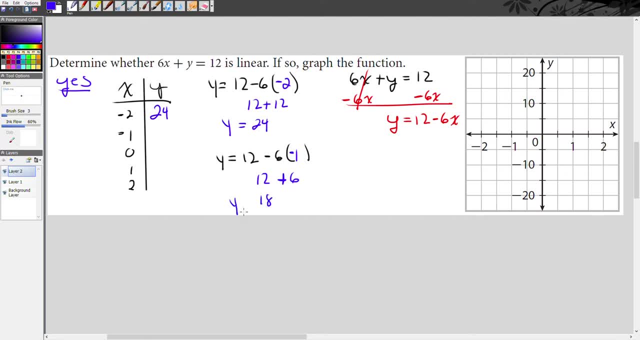 up there, And 12 plus 6 is 18.. So y equals 18 when x is negative: 1. Okay, When x is 0, we got y equals 12 minus 6 times 0. Anything times 0 equals 0. And 12 minus 0 is 12.. 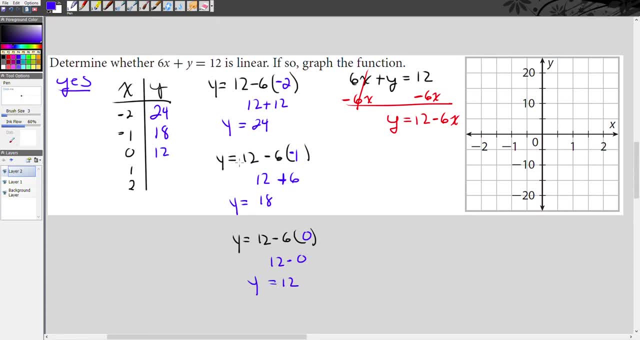 And then Multiplatelets to the left and right: qua lettero is 0,, y is 12.. How about when x is 1?? So y equals 12 minus 6 times positive 1- this time Negative- 6 times 1 is negative, 6.. And 12 minus 6 is 6.. And finally, when x is 2.. So y equals. 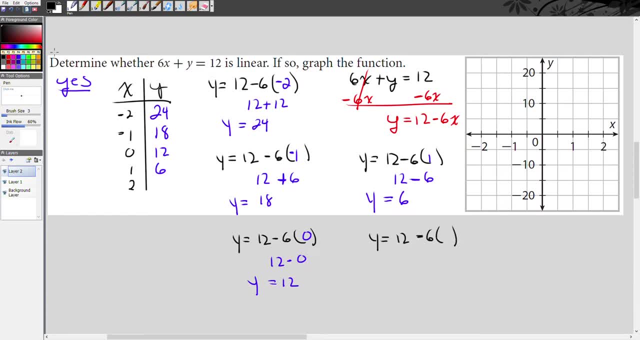 12 minus 6 times 2.. And negative 6 times 2 is negative 12.. And 12 minus 12 is 0.. So when x is 2, y is 0.. So now let's graph this: When x is negative, 2, y is 24.. So here's. 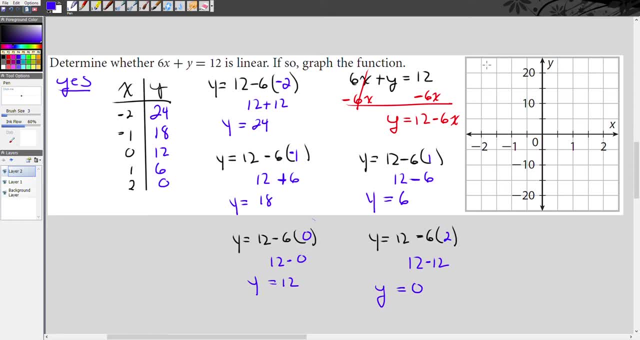 negative 2. 24 is going to be. this would be 25.. So 24 is going to be about right here. When x is negative, 1, y is 18.. Here's negative 1. this is 15, this is 20, so 18, I would say about here. when X is 0, Y is 12 again. 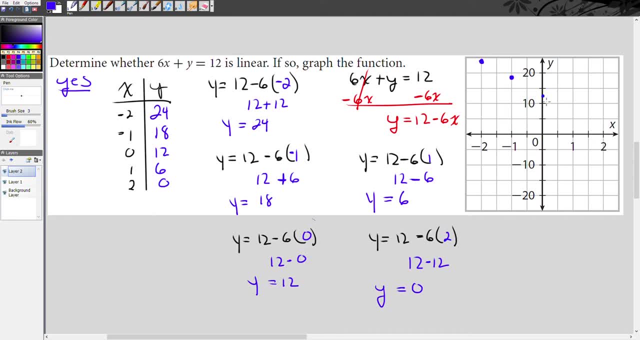 this is 15, so 12 is going to be about here. when X is 1, Y is 6, so here's 1, and this is 5, so 6 is going to be about here. and when X is 2, Y is 0, so here's my. 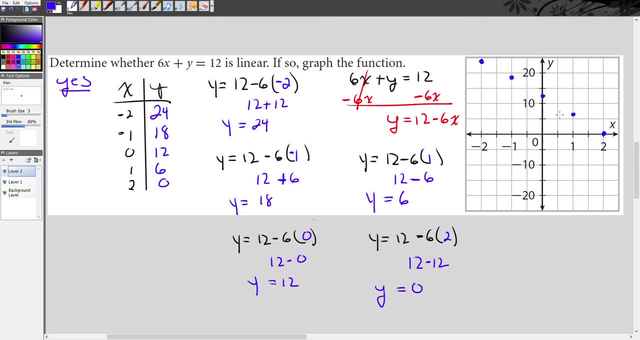 point right here and you can see they kind of line up in a straight line. and there's our linear function. now, when you do this, I want you to use a ruler and draw a straight line all the way through. I don't want to see you know kids doing. 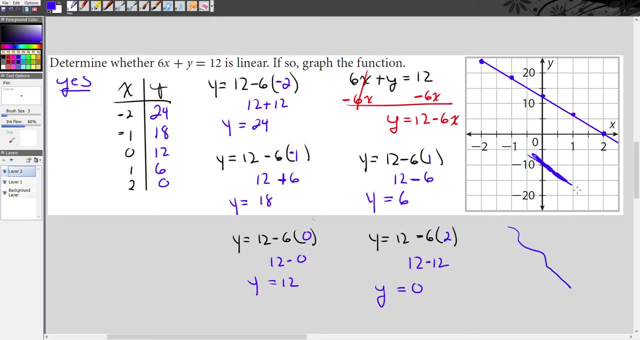 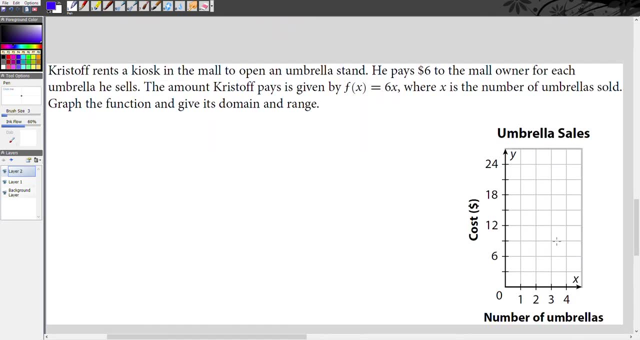 this kind of thing or doing this kind of thing. okay, use a ruler and draw a straight line going all the way through. all right. last part of this lesson: Christophe rents a kiosk in the mall to open an umbrella stand. he pays six dollars to the mall owner for. 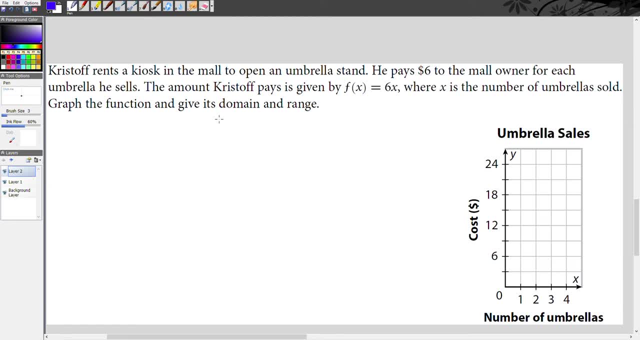 each umbrella he sells. the amount Christophe pays is given by the function. f of X equals 6x, where X is the number of umbrellas sold. graph the function and give its domain and range. okay, so we can look here and we're going to go ahead. 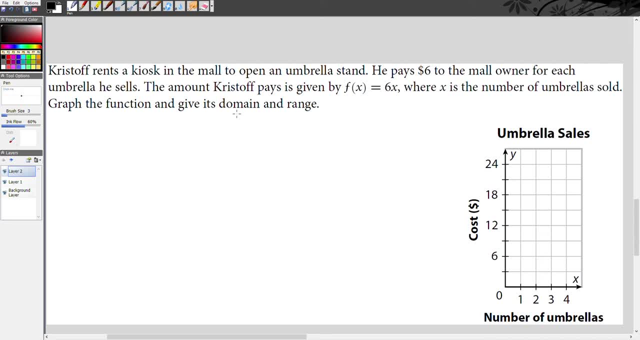 and do. I'm going to follow the same process. so I'm going to say here, you know, X, Y, okay, and we see here zero one, two, three, four. so zero one, two, three, four, and we're going to substitute these values for X. this is kind of easy, so we could kind of do this mental math, right. 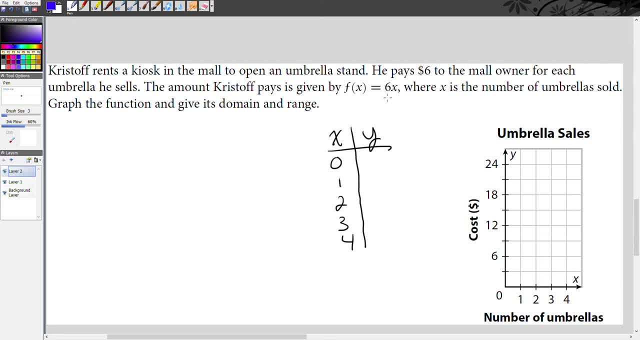 so when X is 0: 6 times 0 is 0, so Y is 0. when X is 1: 6 times 1 is 6. when X is 2: 6 times 2 is 12. when X is 3: 6 times 3 is 18, and when X is 4: 6 times 4 is 18 and. 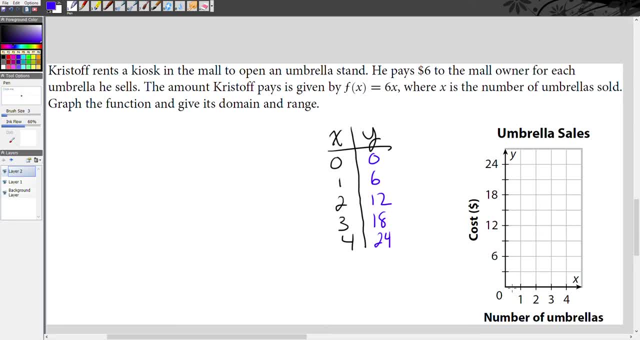 24, so we'll grab these points. we have 0 comma 0, 1 comma 6- it's right here- and 2 comma 12 is here, 3 comma 18 and 4 comma 24.. now would I draw a line to connect. 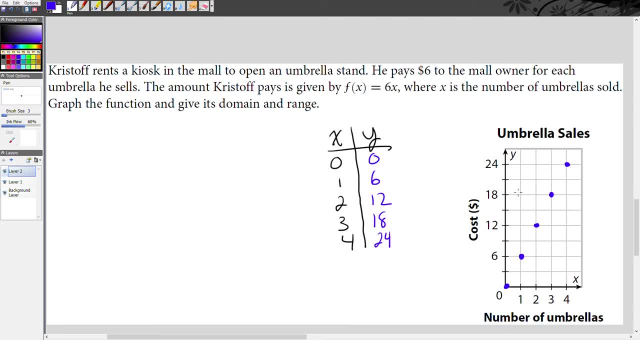 these. well, in this case, I actually wouldn't draw a line to connect these because, if you remember, we learned about a concept called continuous and discrete data. continuous data is where all the data connects, like time or temperature or distance. everything connects, but here we have umbrella sales, so you're either